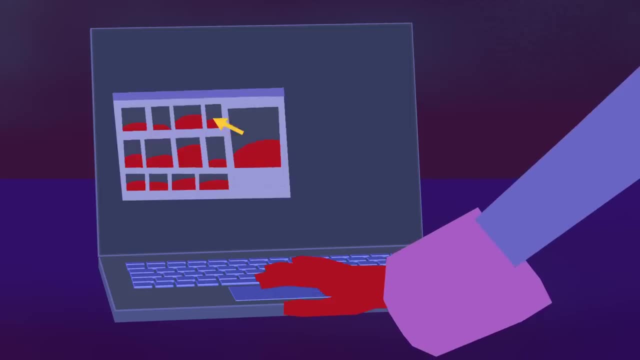 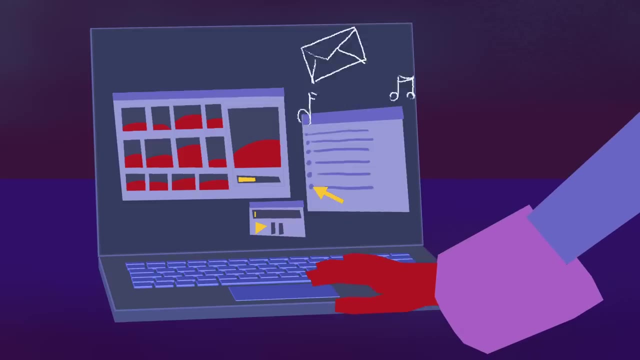 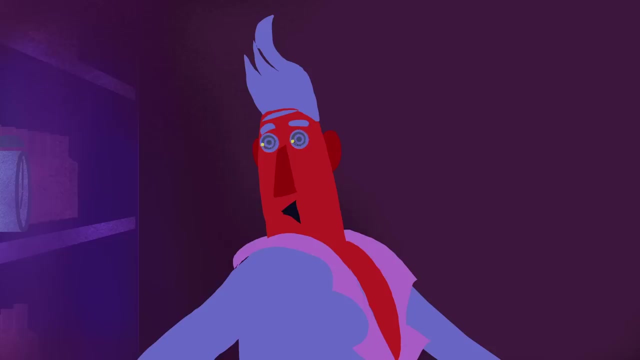 and what to switch to Done right. computers move so fluidly between their various responsibilities they give the illusion of doing everything simultaneously, But we all know what happens when things go wrong. This should give us, if nothing else, some measure of consolation. 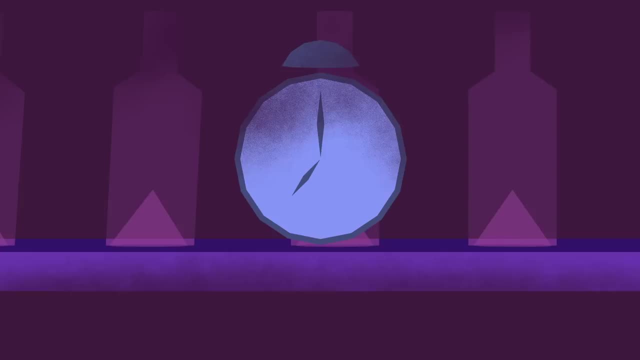 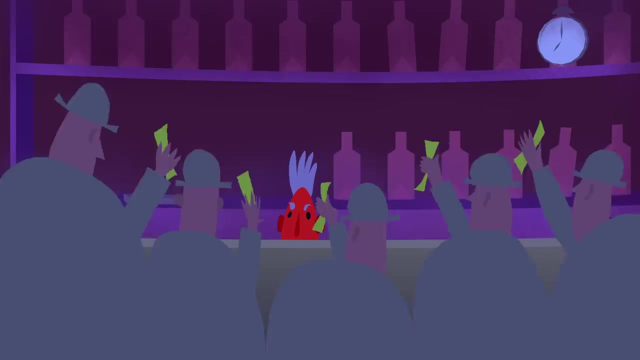 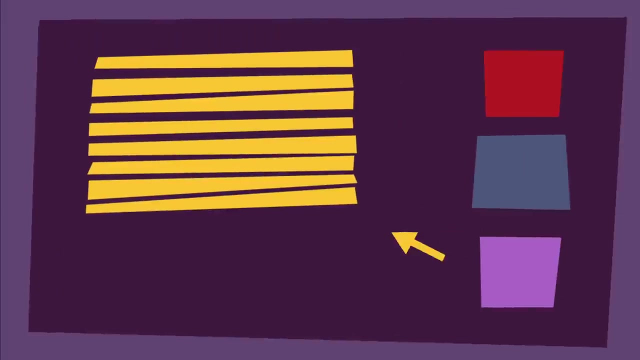 Even computers get overwhelmed sometimes. Maybe learning about the computer science of scheduling can give us some ideas about our own human struggles with time. One of the first insights is that all the time you spend prioritizing your work is time you aren't spending doing it. 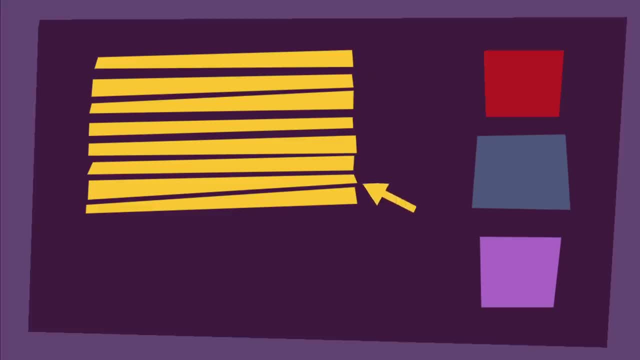 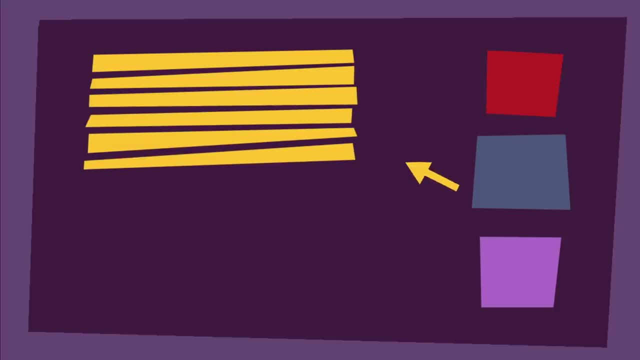 For instance, let's say, when you check your inbox, you scan all the messages, choosing which is the most important. Once you've dealt with that one, you repeat- Seems sensible, but there's a problem here. This is what's known as a quadratic time algorithm. 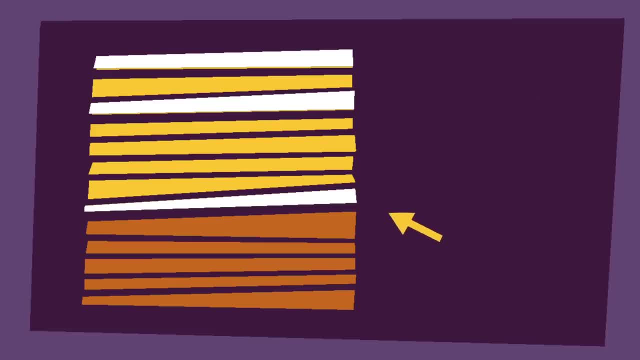 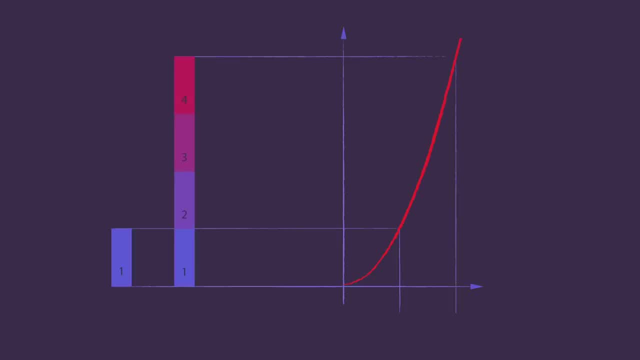 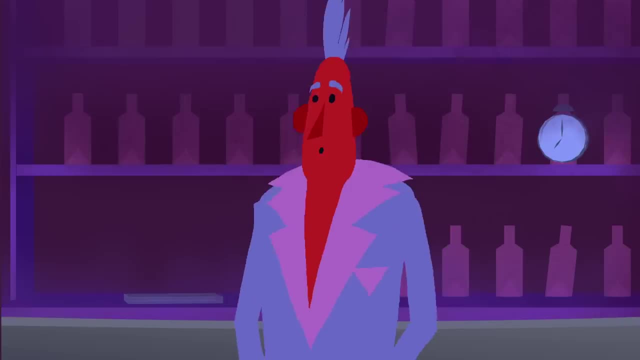 With an inbox that's twice as full. these passes will take twice as long and you'll need to do twice as many of them. This means four times the work. The programmers of the operating system Linux encountered a similar problem in 2003.. 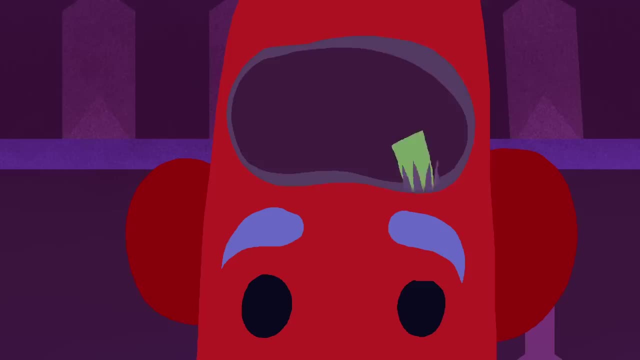 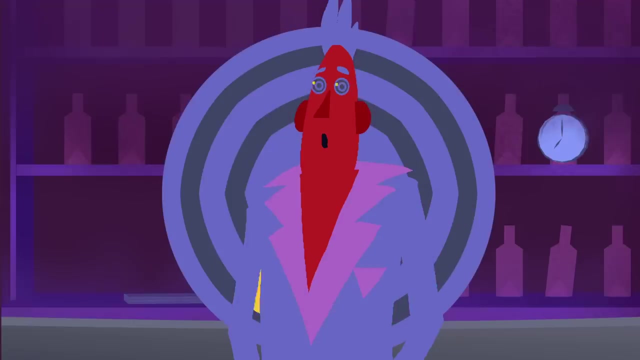 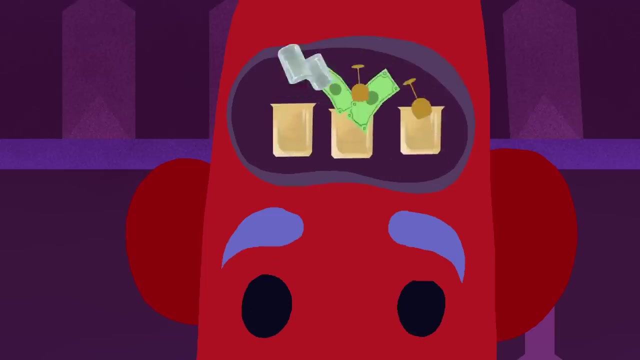 Linux would rank every single one of its tasks in order of importance and sometimes spent more time ranking tasks than doing them. The programmers' counterintuitive solution was to replace this full ranking with a limited number of priority buckets. The system was less precise about what to do next. 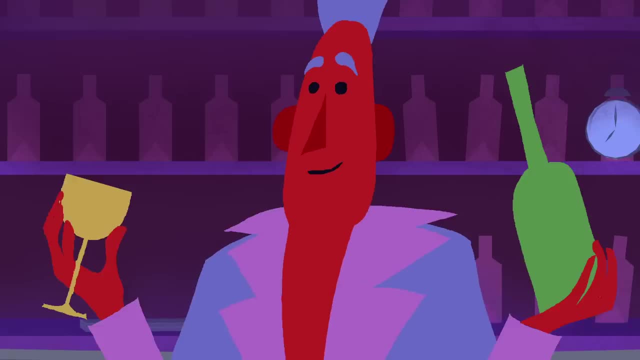 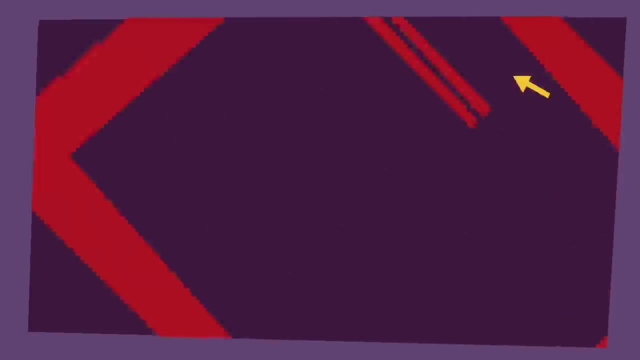 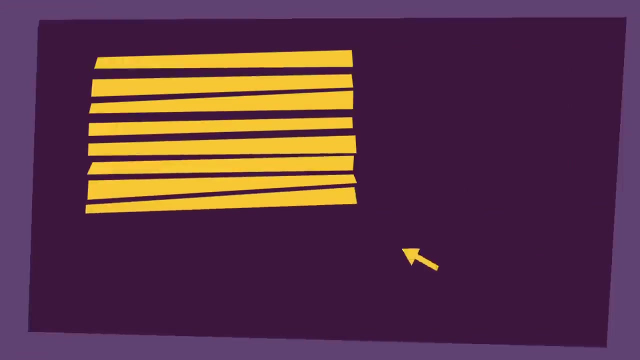 but more than made up for it by spending more time making progress. So, with your emails, insisting on always doing the very most important thing first could lead to a meltdown. Waking up to an inbox three times fuller than normal could take nine times longer to clear. 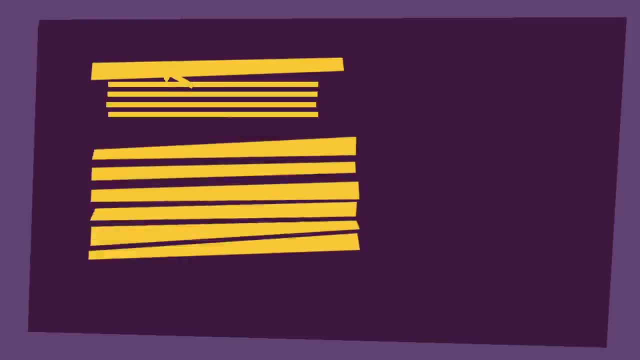 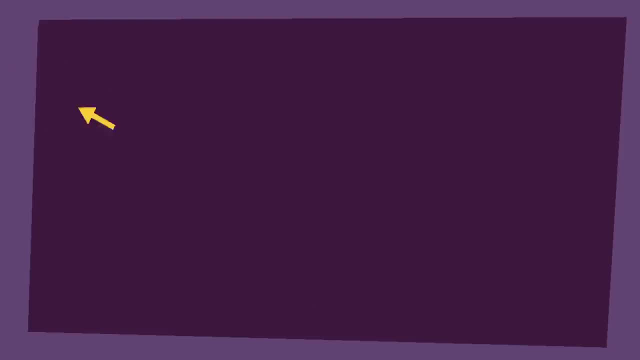 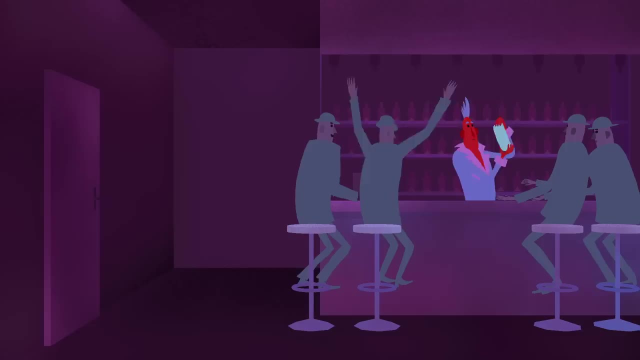 You'd be better off replying in chronological order or even at random. Surprisingly, sometimes giving up on doing things in the perfect order may be the key to getting them done. Another insight that emerges from computer scheduling has to do with one of the most prevalent features of modern life. 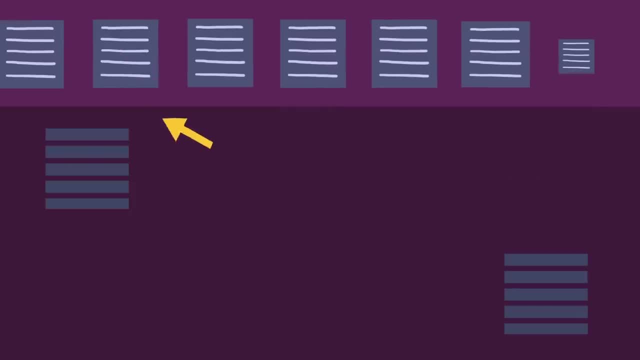 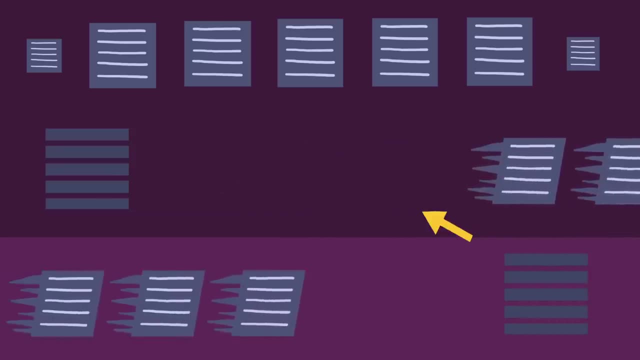 interruptions. When a computer goes from one task to another, it has to do what's called a context switch: bookmarking its place in one task, moving old data out of its memory and new data in. Each of these actions comes at a cost.